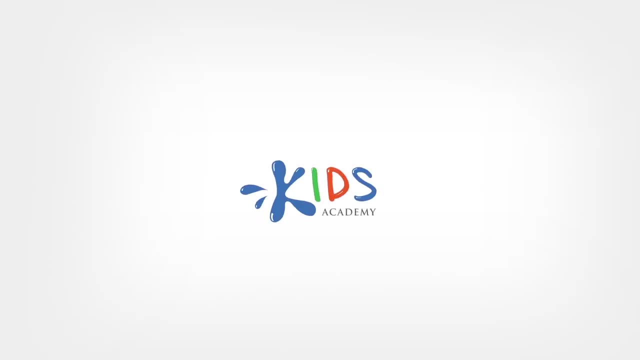 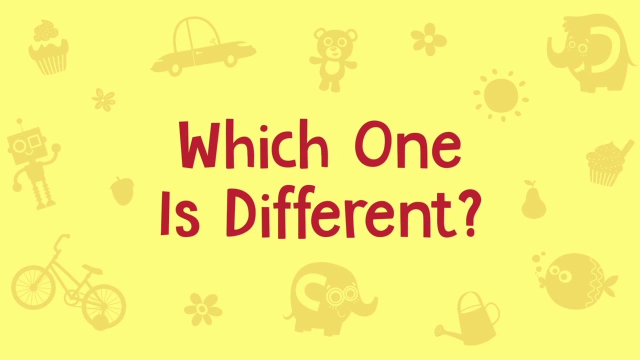 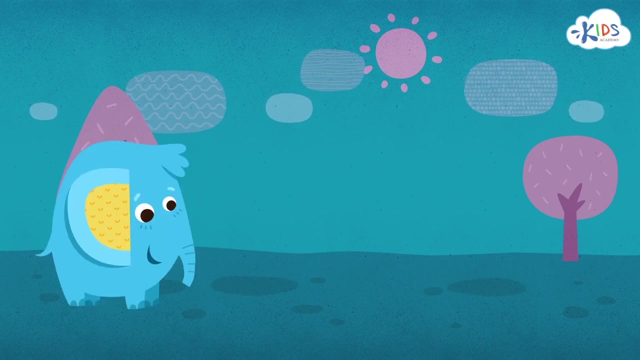 Hello boys and girls. Today we're going to find objects that are just a little bit different than the other ones in the group. Let's take a look at our friend Billy. Billy is an elephant, He's cool, he's smart and he really likes peanuts. What color is Billy? Billy is blue. 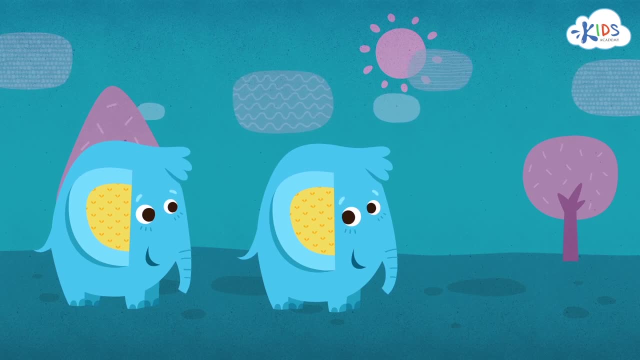 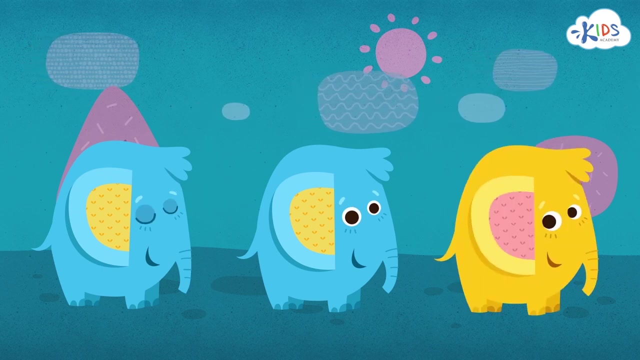 Whoa, Look at that. Another blue elephant, just like Billy. It's the same size, same color and the same type of animal. They look exactly the same. Oh, my Another elephant. This one looks just like the others. Is it exactly the same as the other elephants? No, 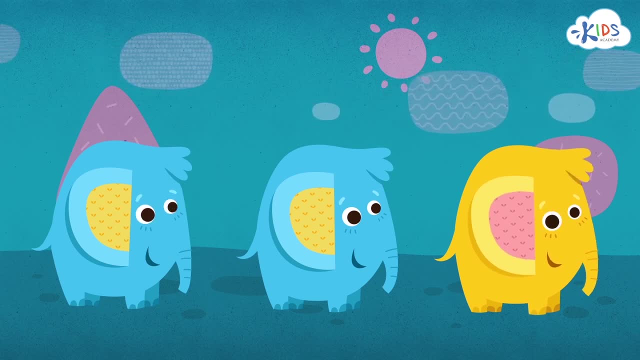 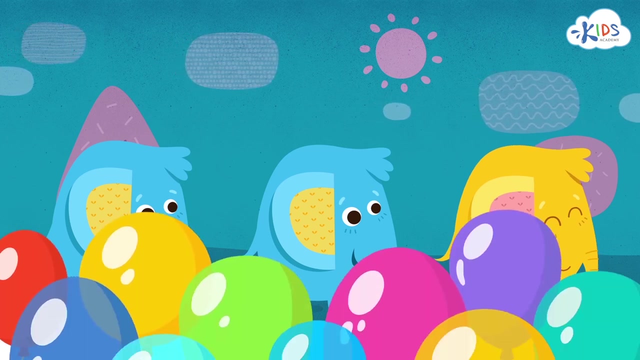 This elephant is the same size and the same type of animal, but this elephant is yellow and the other ones are blue. The color is different for this elephant. This one is the one that is different. Before we get started, let me give you some hints, so you 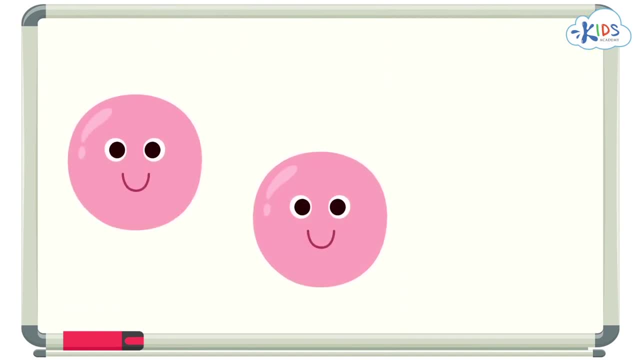 know what you can look for. Some things to look out for are color: Like is one of the colors different from the others. See, this one is a different color. Shape: Like is one of the objects a different shape than the others. See, this one is a different shape. 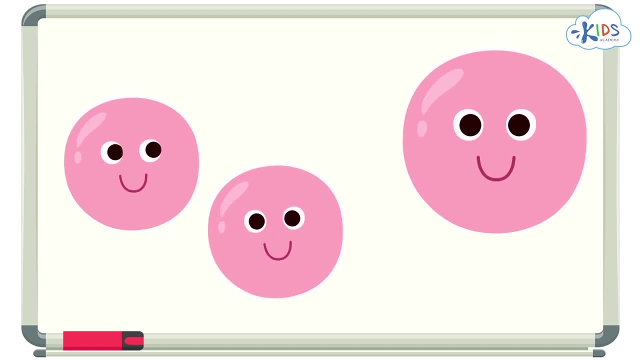 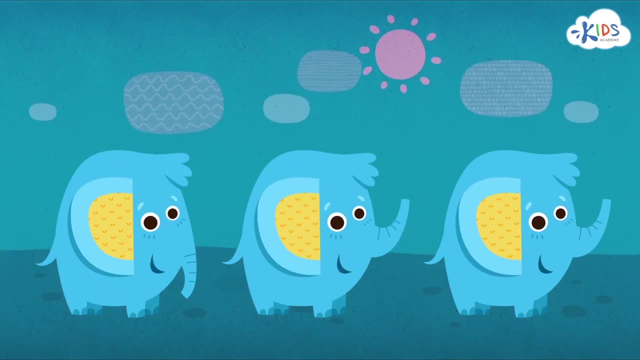 Like. is one of the objects larger or smaller than the others? See this one is a different size And position. Are all of the parts of the objects in the same position or pointed in the same way? See this elephant has a trunk facing down and the other elephants. 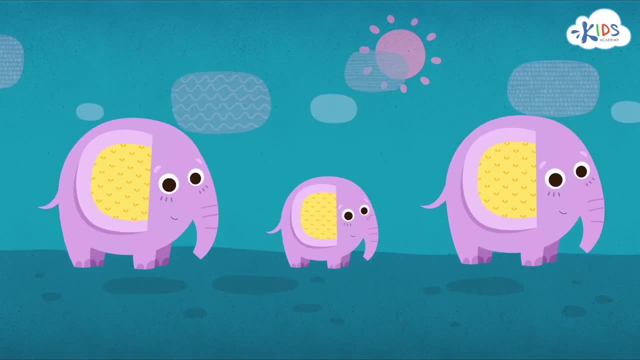 have their trunks facing up. Let's look at some other groups of objects and see if we can find the one that just looks like the other one. Let's look at some other groups of objects and see if we can find the one that just looks.